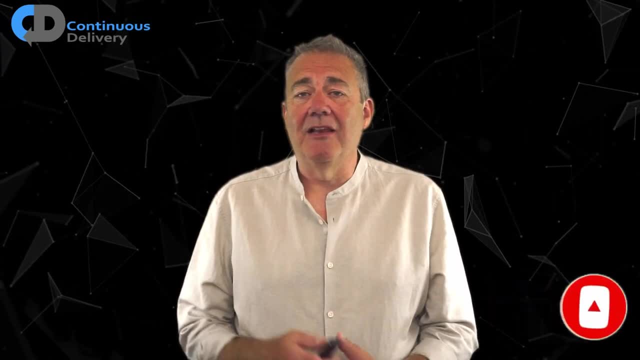 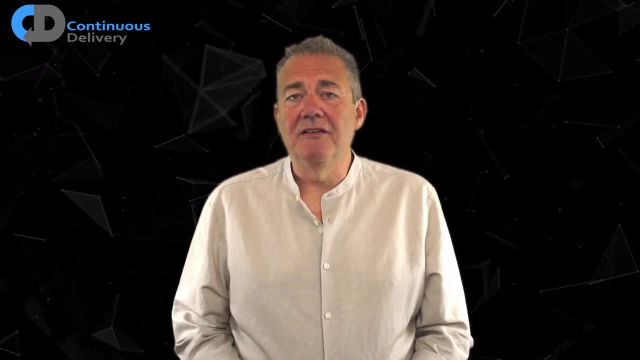 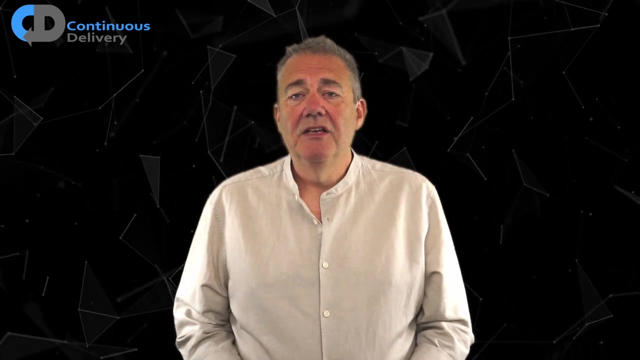 haven't already, please subscribe and if you like, the video hit like Today. I'd like to try something a little bit different. I want to do an exercise in working with some existing code. I'd like to demonstrate some of the techniques of improving existing code and the application of a simple four-step. 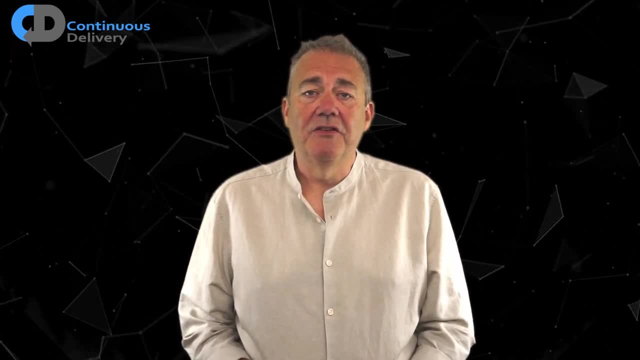 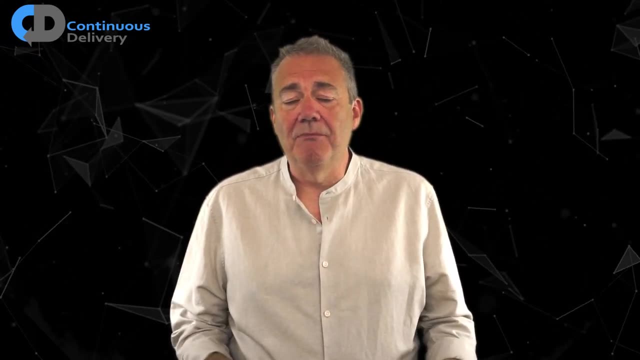 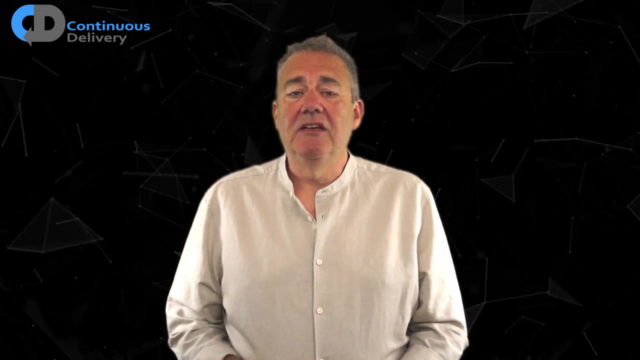 process that I tend to use myself when I'm working in those kinds of environments. I'm going to cover all of this in a few separate episodes, so I'm going to create this little mini series of linked videos to allow me to explore this in a little bit more depth than I would normally cover in a 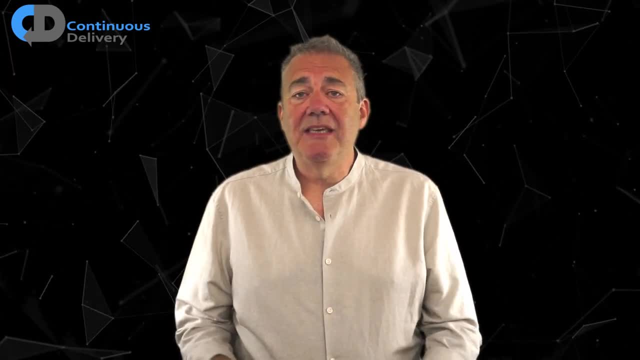 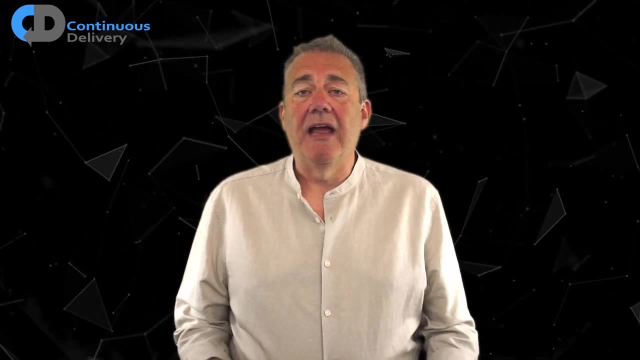 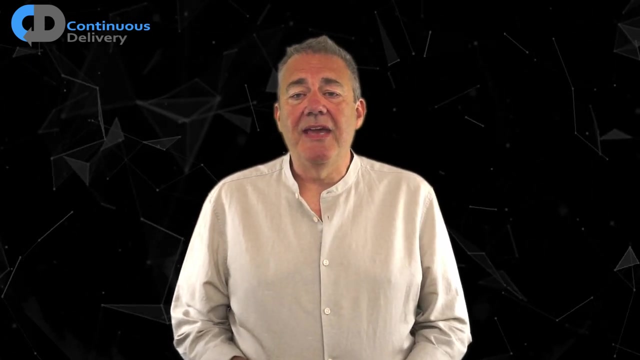 video. So where do we start? Where do we begin with such things? Well, I started by going and doing a search on the internet for bad code and I found some, So we're going to start with some fairly poorly organized code. The code that I picked is: 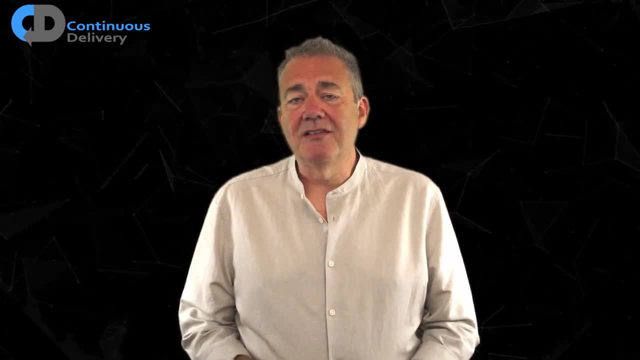 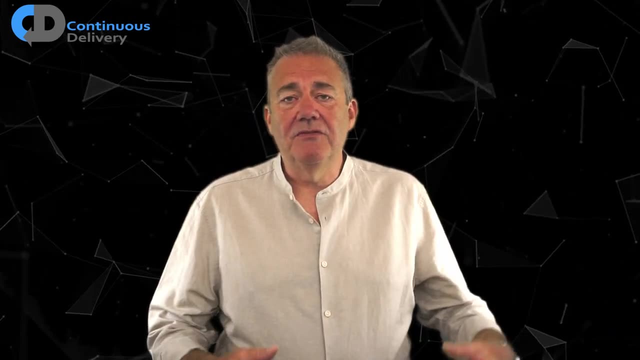 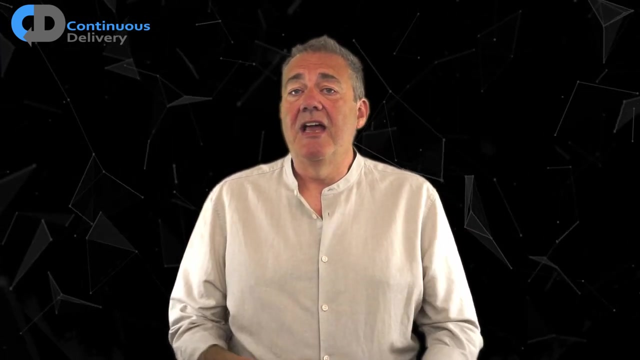 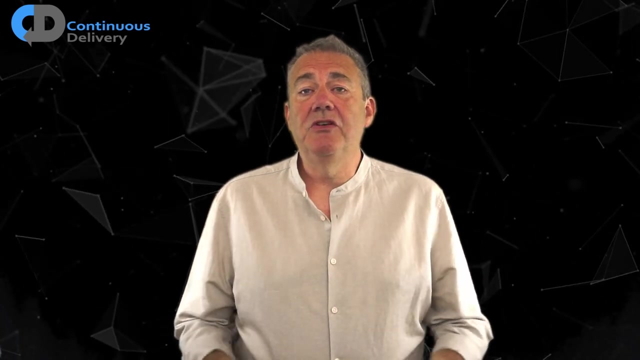 pretty nasty. It's focused on traffic. I'm not going to translate it into some JSON. I'm going to try and keep the code working and make it better as part of my efforts. So I recorded me working through this bad code and refactoring it. I'm going to release this as a series of 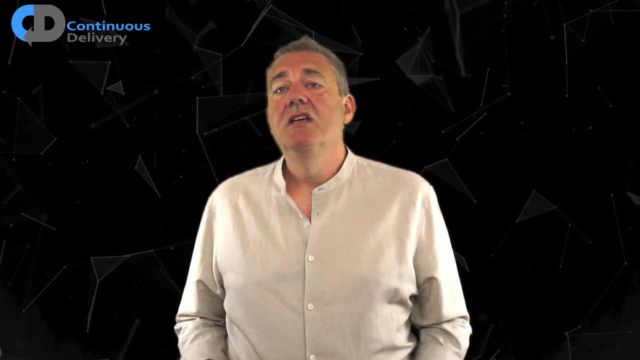 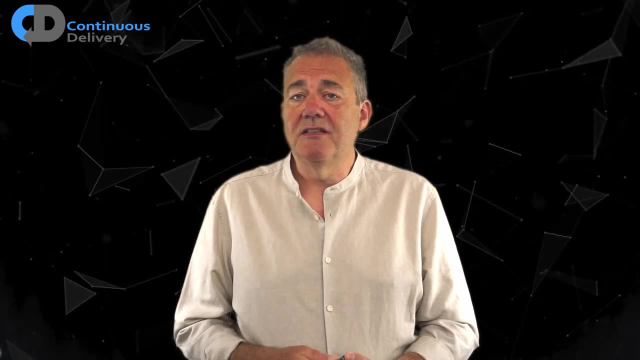 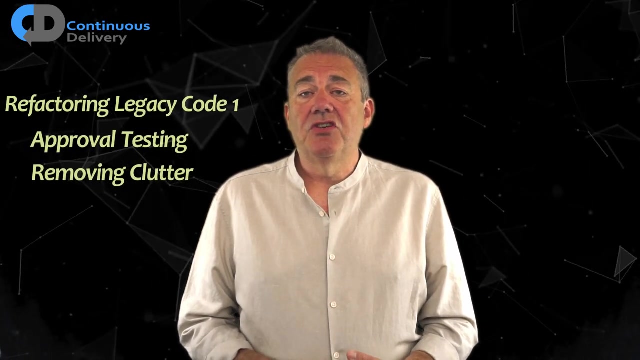 videos. I'm going to do three edited videos that highlight different aspects of the work, and I'm going to release the whole thing from end to end for those people that would like to see the whole process. The first in this mini-series focuses on two things: approval, testing and removing. 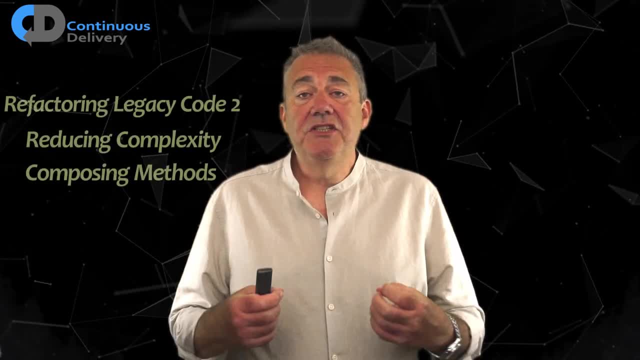 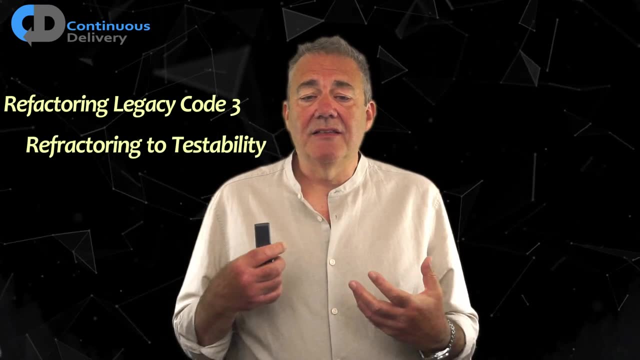 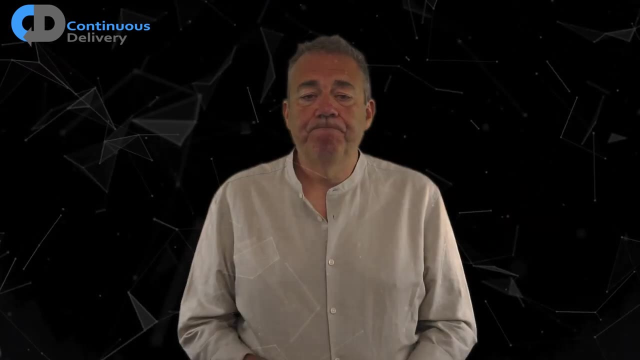 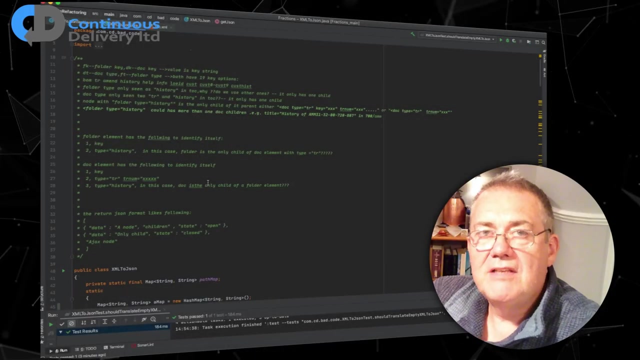 clutter, The next will cover reducing complexity and composing methods, and the last in the series will look at refactoring to testability, And then we've got the whole video, which will release some other way. One of the techniques that I fairly recently adopted is one called approval testing, and I 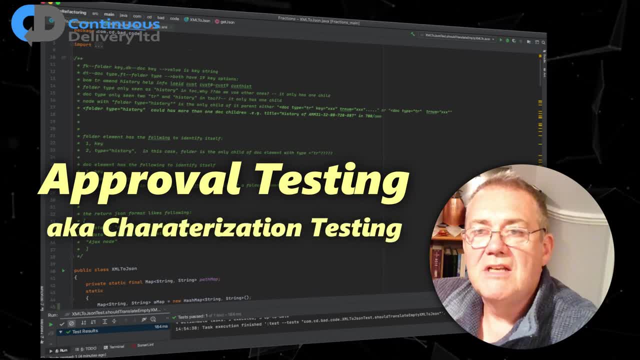 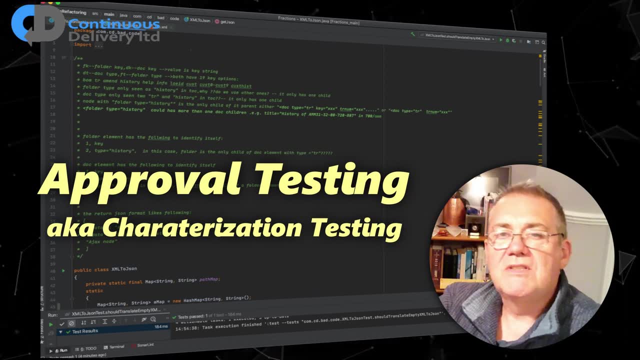 must admit that the first time that I heard about approval testing, I was a bit dismissive of it, and that was my bad. I misunderstood the context in which I was talking about approval testing. Approval testing makes sense, at least because approval testing is a great tool if you use it in 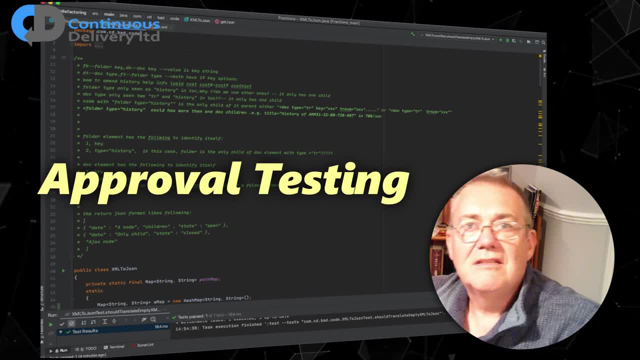 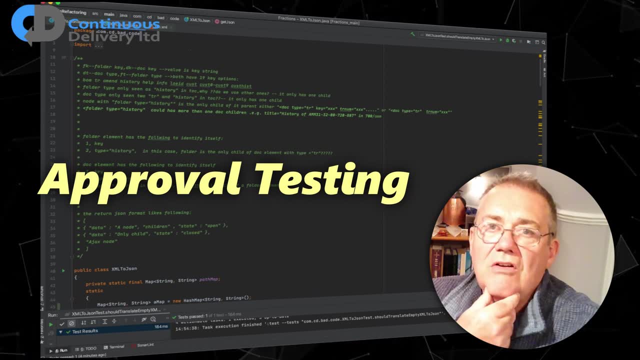 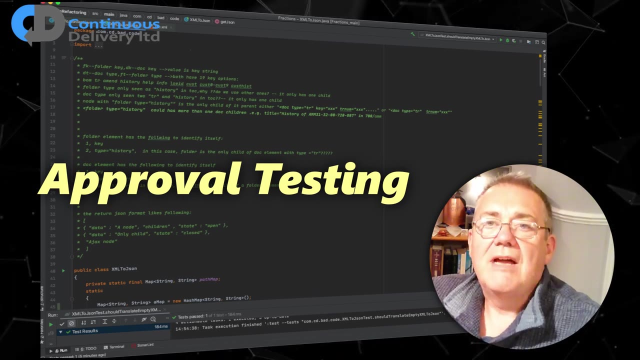 the right context, and that context is exactly this: When you've got a body of existing code and you'd like to safely change that code without changing its behavior- which is what refactoring is- then how do you do that? What sorts of tests can you create that allow you to do that? And 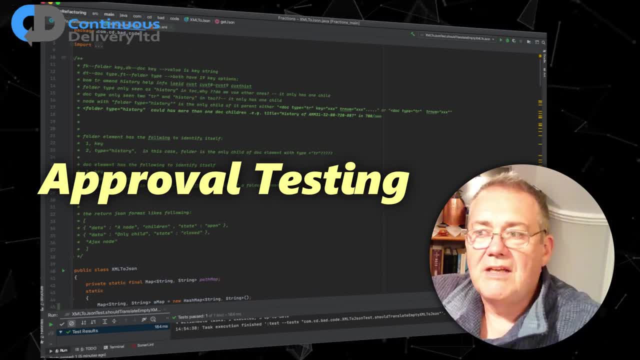 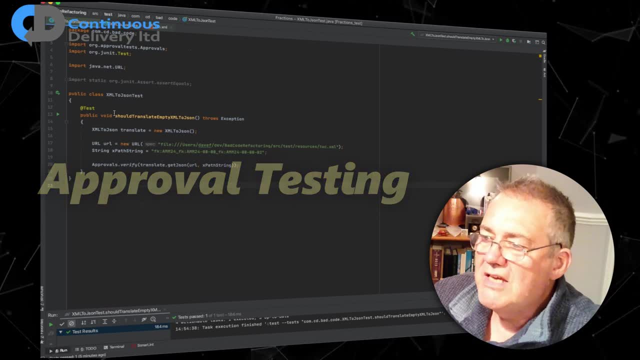 approval testing allows you to do that- create those sorts of tests quickly and efficiently. So I've started off by building the outlines of such an approval test. So here's my test. I've got one test case at the moment. should translate empty XML to JSON, which is: 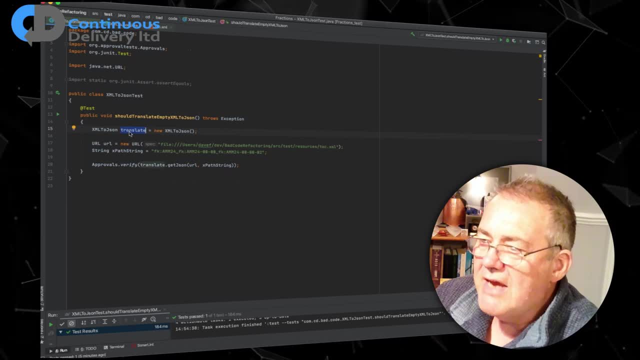 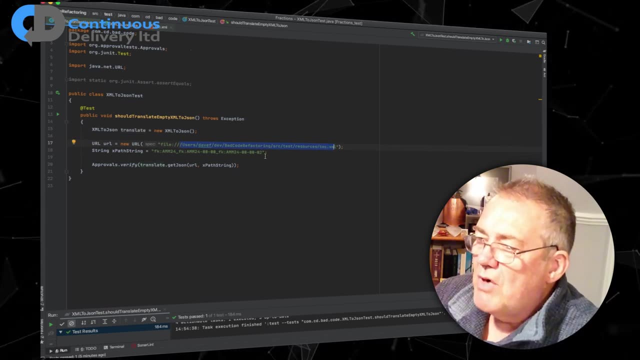 basically just saying what the whole piece of code does. So I'm going to create an instance of the class, the XML to JSON class. I'm going to supply it with some appropriate resources. So this is a search key that's mentioned in one of the comments. 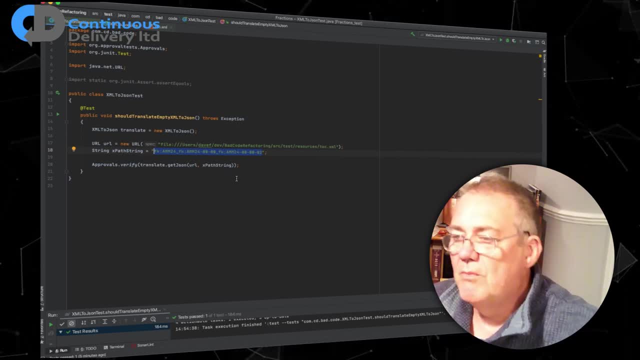 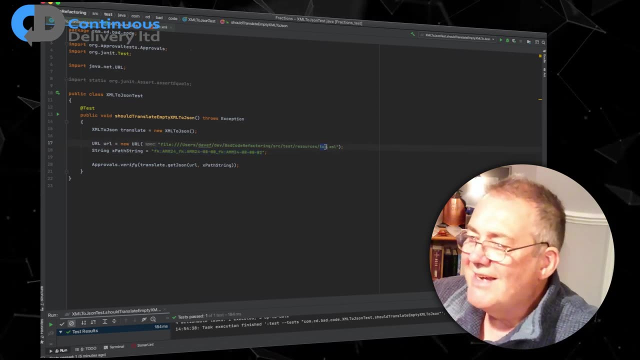 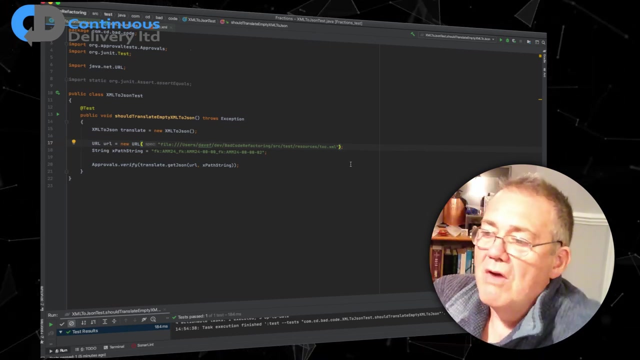 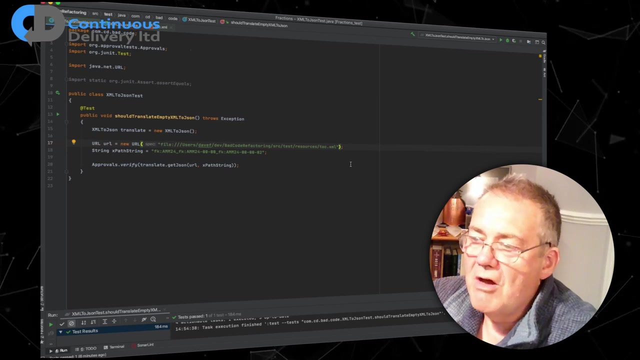 As an example, there's a main method in the block of the code that's used as a test, So I just ripped this out and copied that. I didn't have access to the original XML file that this code was tested with, So I've created my own. from what I could interpret from the comments in the code, This is: 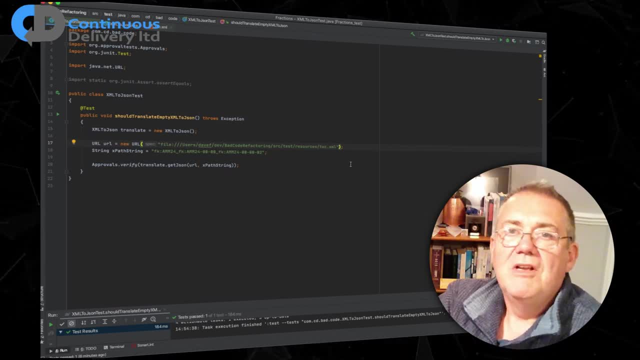 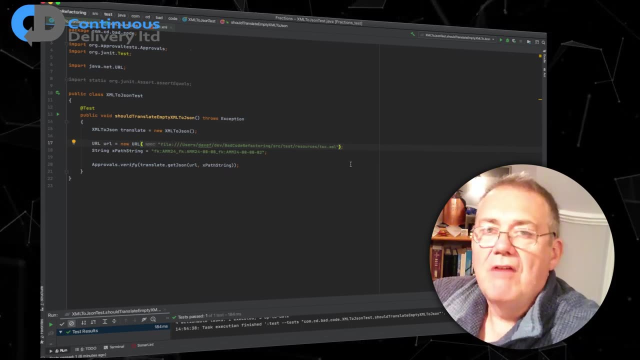 a bit ironic, because usually I recommend that people do try to avoid comments in code. In this case, I've actually relied on them. In this case, though, I've kind of got these input parameters and I've got these to a stage where they're giving me a certain level of coverage in the test. So if I run this approval- 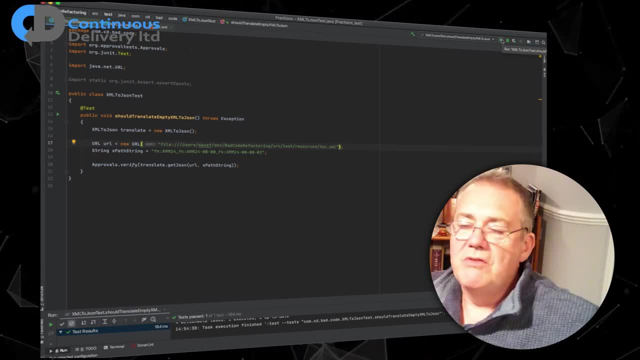 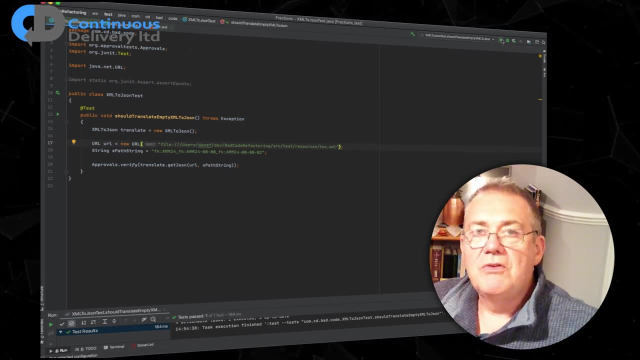 test now. So sorry, I should explain the way that approval tests work. So what happens when you're in an approval test is it just captures the output from the code that you call, Whatever, whatever it is that you call, In this case I'm calling get JSON. 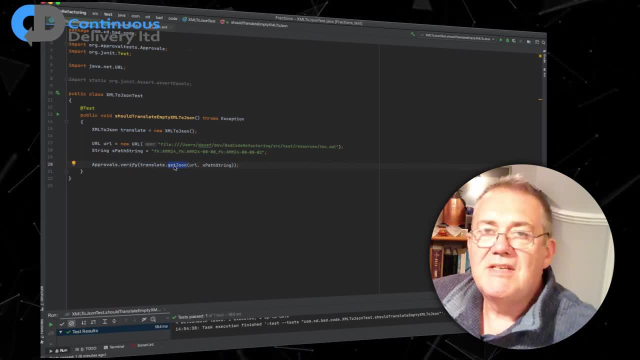 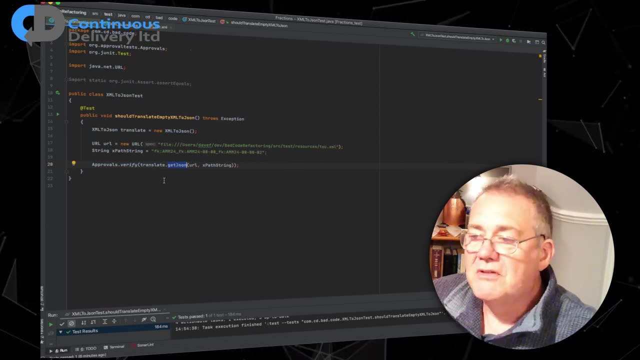 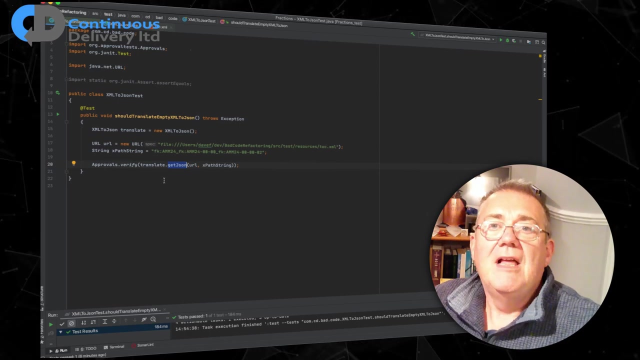 the method. This is the method. This is the public method that we'll be testing on this class with my test parameters, And when I call the get JSON method, I'm going to get a result. What you do with the first time you run an approval test, that test will fail, But what you can then do is that. 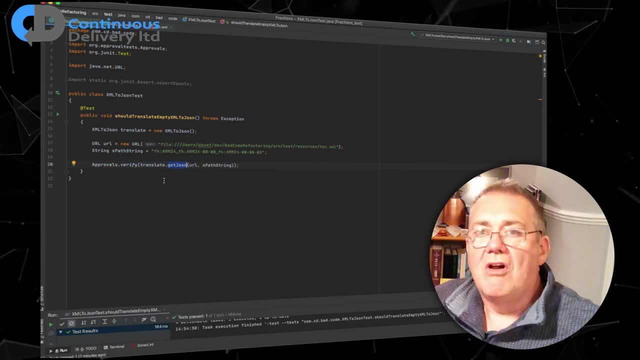 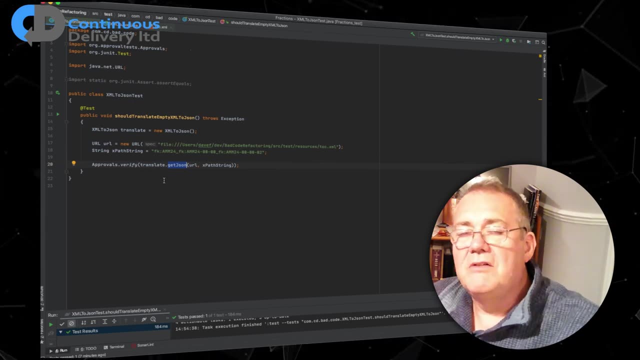 you can save. you can save an image of that result to disk And then subsequently, every time that you run the approval test, it's going to open the code again- generate the results again and just do a straight comparison between the, the version that you saved and the version that you've just generated in the context of this test. 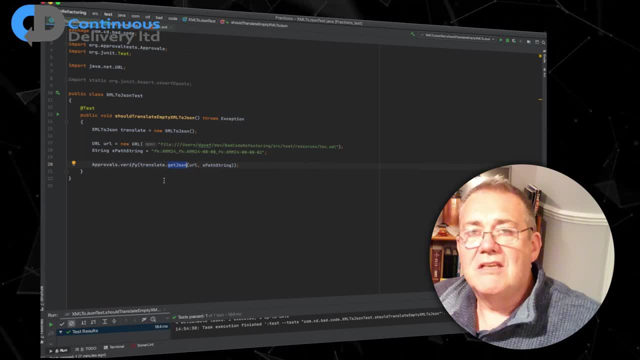 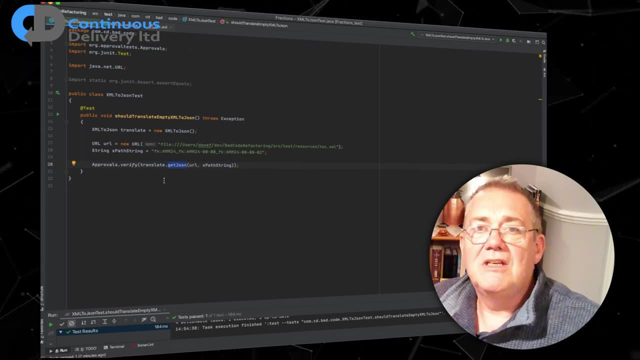 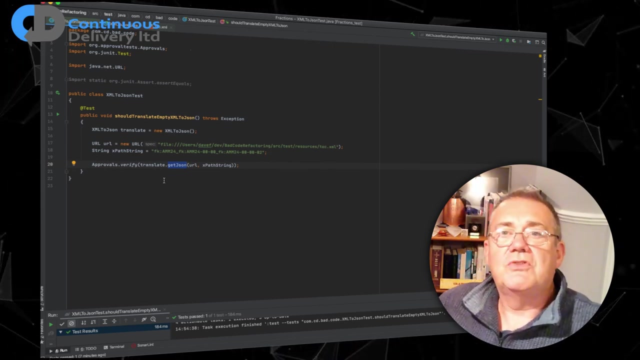 As long as the output remains the same, the test will pass. You have approval. If you make a change and it disrupts that, it stops the code doing what it was doing before. the test will fail and inform you of that fact. So it's a very, very useful tool when you're doing. 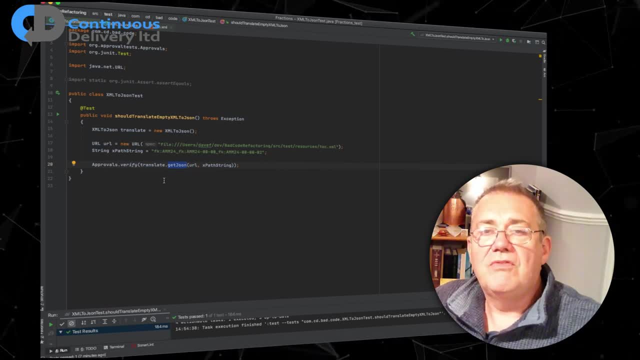 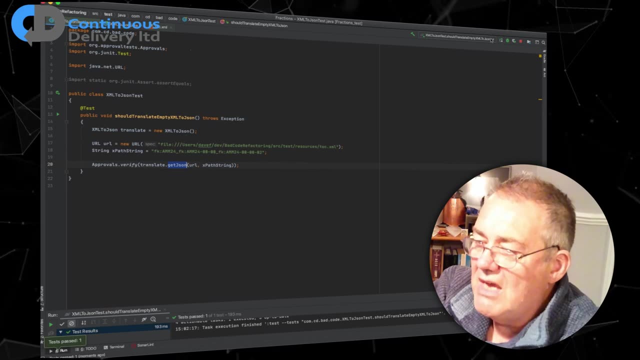 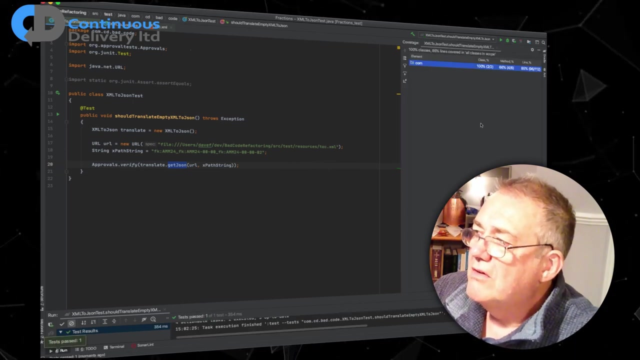 factoring, where the whole point is to avoid changing the behavior of the code, at least at this stage. So if I run my approval test now, I've already saved the image and my test passes, so that's all good. The other thing that I can usefully do is that I can run the approval test. 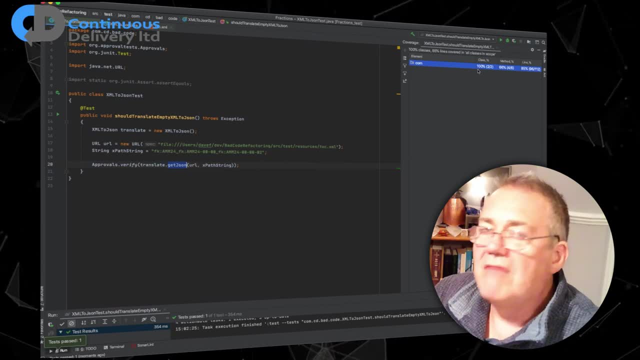 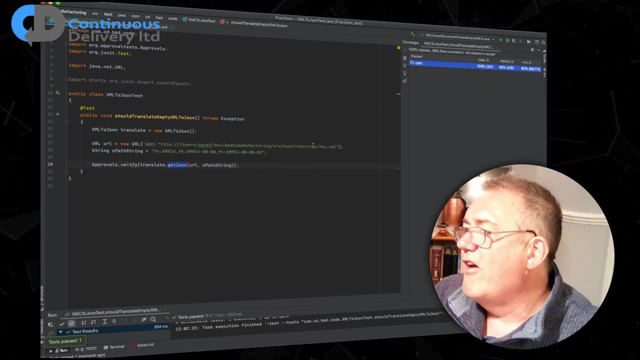 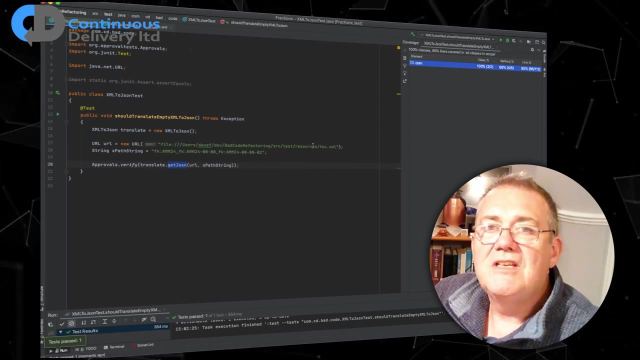 with coverage And I can see that at the moment, the level of line coverage and method coverage that I have, I've got 66% of methods but I'm only covering 85% of the lines of code. If that's all I could get, I would feel reasonably confident in still proceeding. 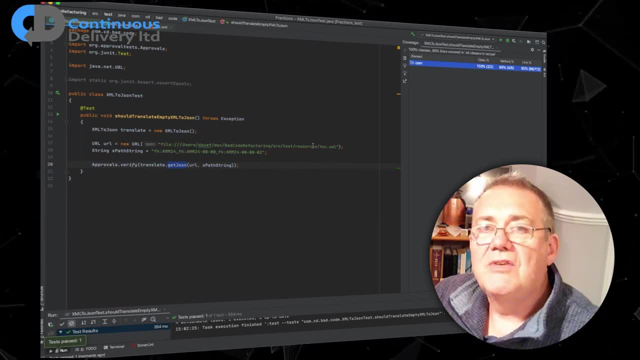 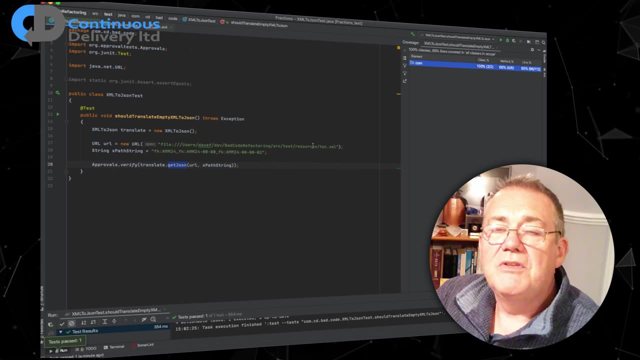 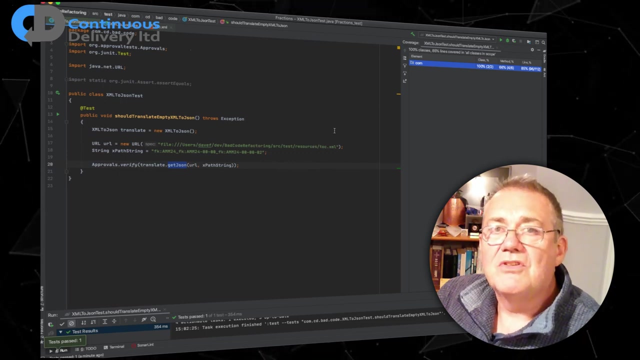 using very cautious refactoring techniques to make changes to this code base with that level of protection. To be honest, there are some refactorings that I will do in a code base without any tests, because I'm confident in my ability to make those sorts of changes without. 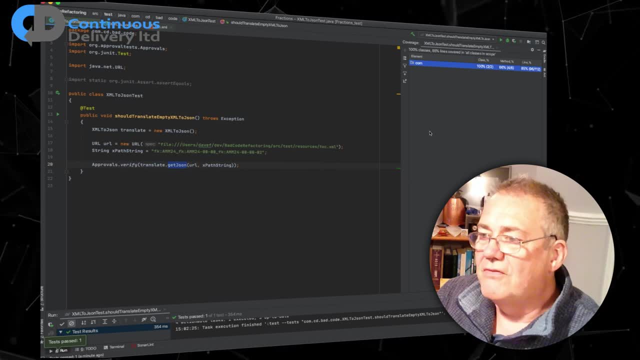 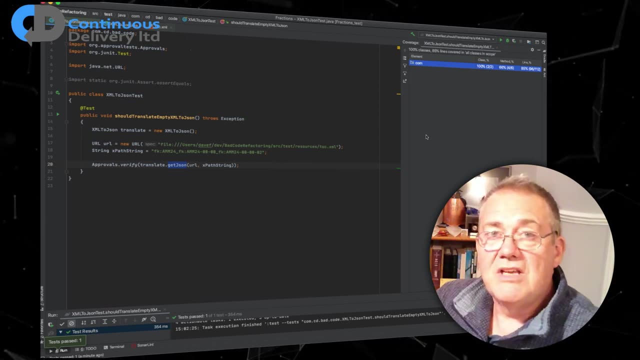 breaking things. But having the test is a great, great defense and gives you a much higher level of confidence that you can proceed and carry out more risky changes to the code, as we'll see as we go through this exercise. So we can dig in and we can see what that means in. 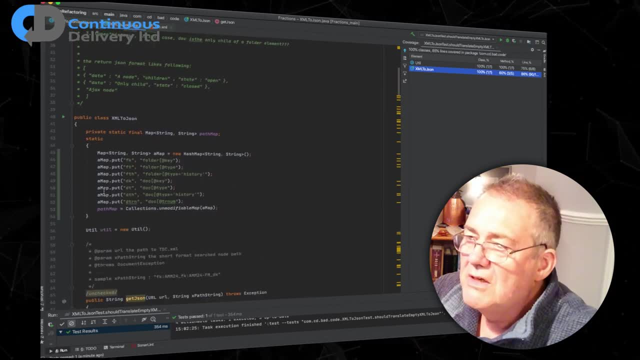 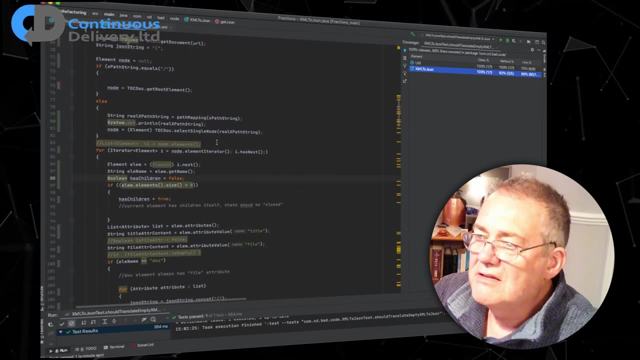 terms of the coverage in the code. So here's my code, And where there's a little green bar on the side here, it means that the test covers that case And there's a line here. So if the XPath string doesn't begin with a slash, 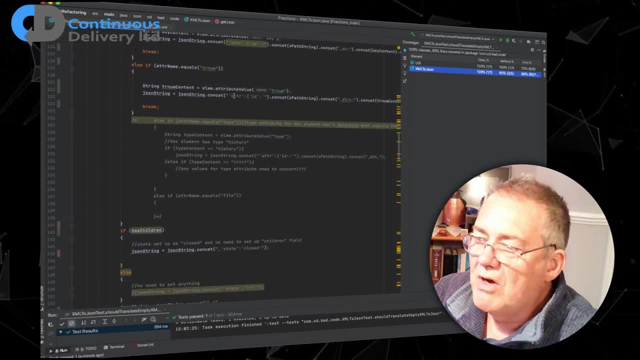 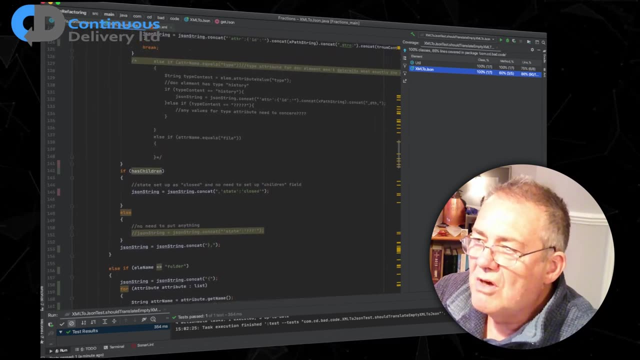 it finds the root node. That's not a very risky thing in my mind to test. There's some commented out code here And that block because it's all commented out. maybe there's a bit more. Yeah, there's not much going on there. 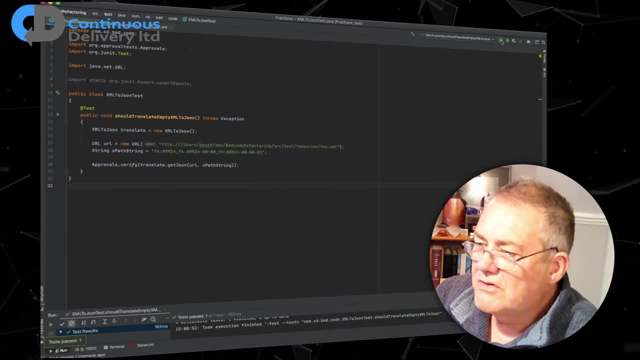 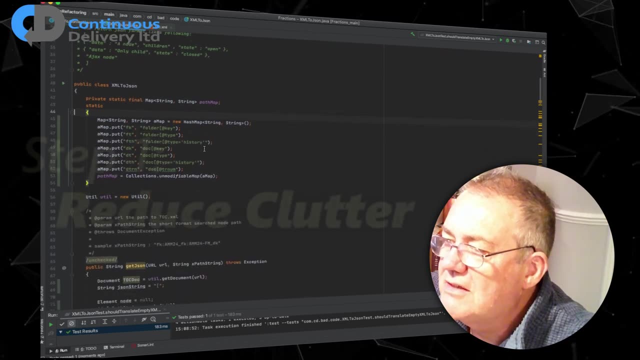 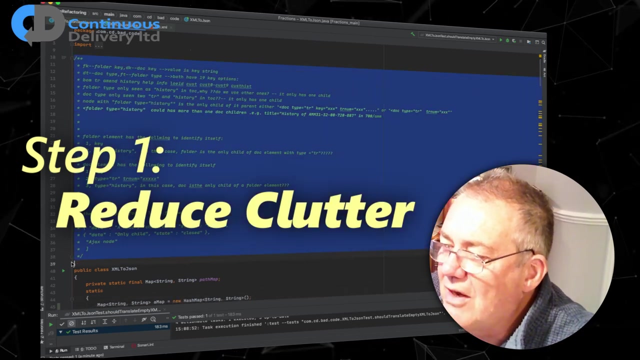 So here's my test, And that's giving me a certain amount of confidence to be able to make some progress. So I think the first step in refactoring these things is let's just get rid of some of the data. I'm going to leave some of the comments that seem like they might be useful. I'm trying. 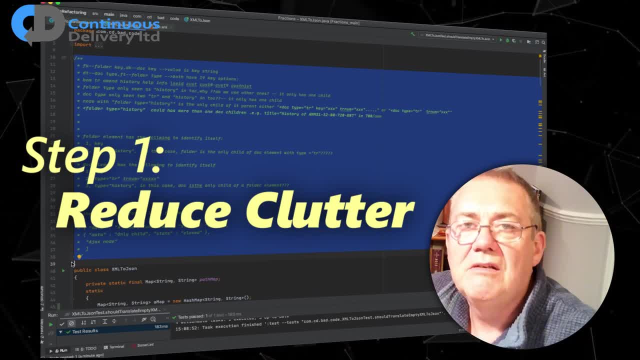 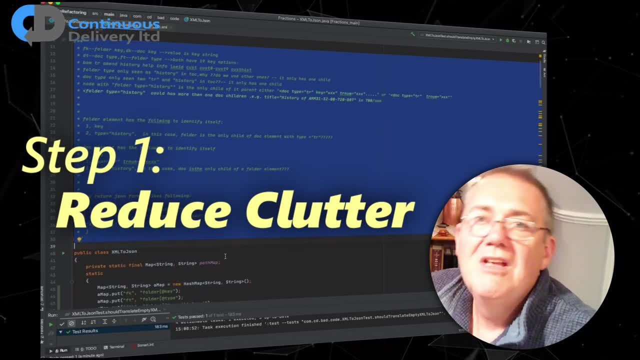 to do this as though it's a. I'm trying to behave as though I'm really doing this in a real production situation, And so I'm going to be somewhat cautious in terms of moving forward. But you've also got to have a degree of courage and confidence. You've got to be able to take some 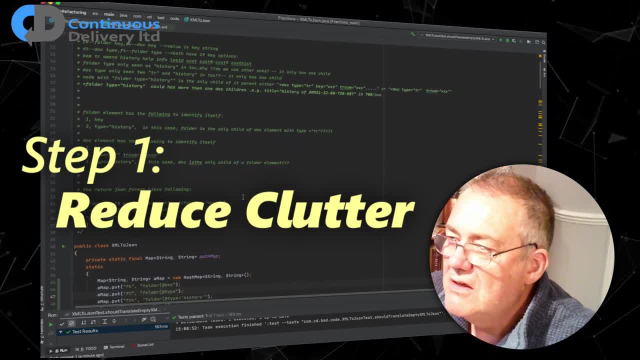 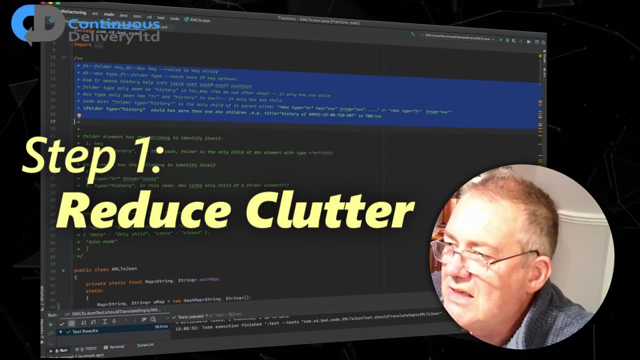 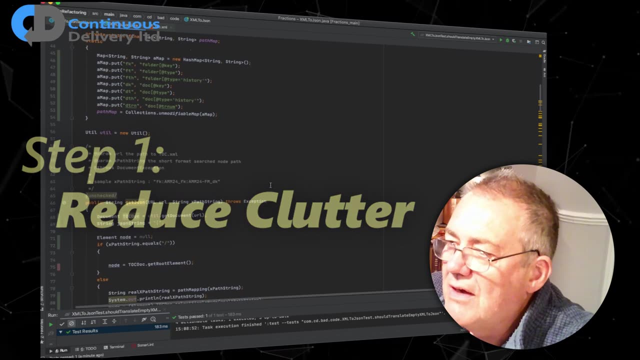 chances along the way with some of this stuff. So first looking at these, there's an awful lot of stuff that I'm not very interested in here. It's really not telling me very much. I'm going to leave this for now and come back to this, This thing. 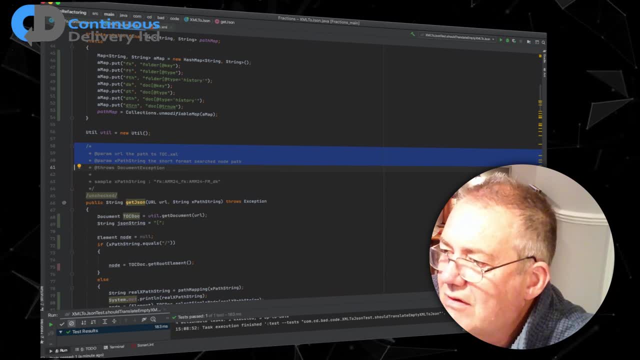 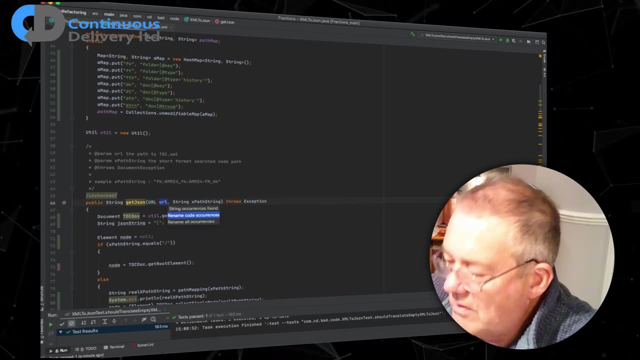 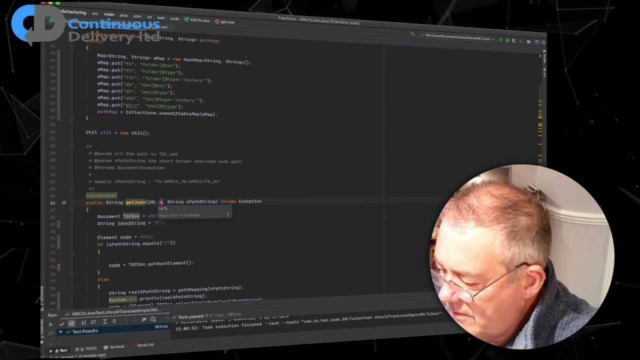 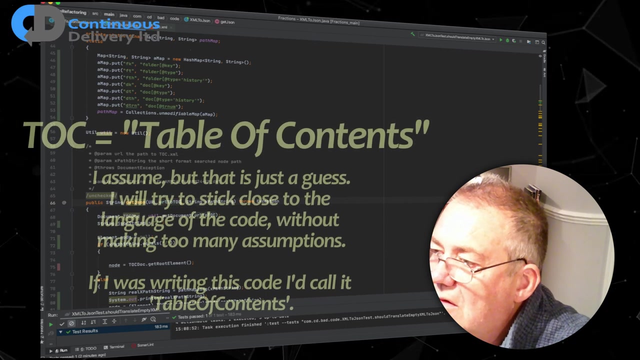 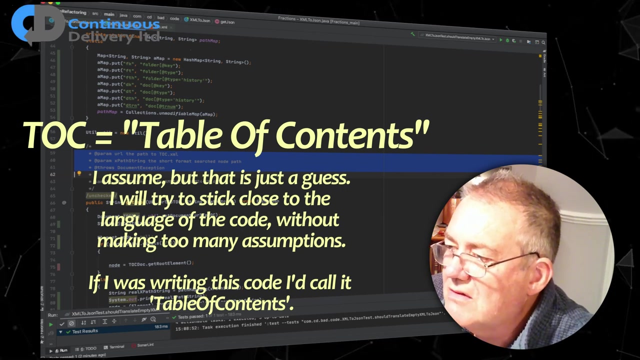 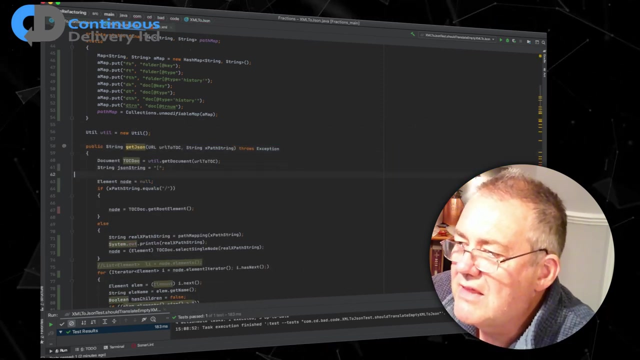 so the parameter of the URL path to. so if we were to rename this variable to URL to TOC, which is what the document's called, that kind of eliminates the need for this. All of the rest of this stuff is just waste. It's not telling us anything, So that can go. 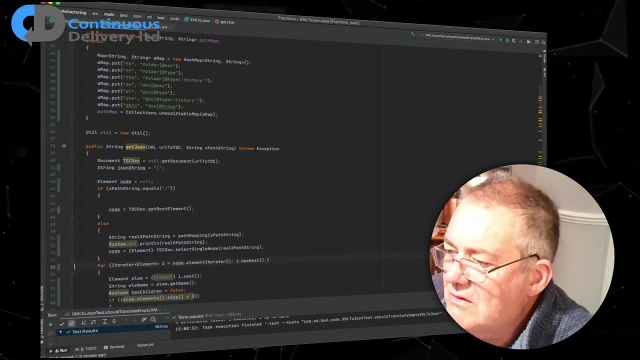 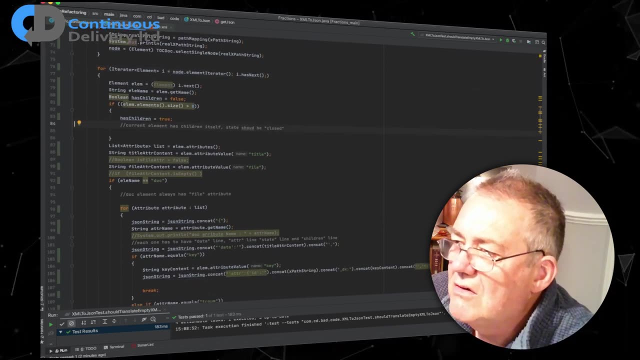 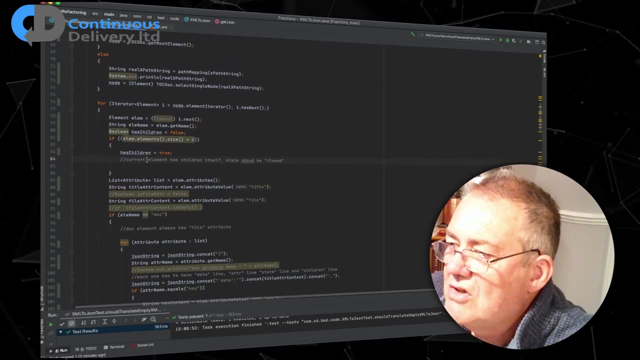 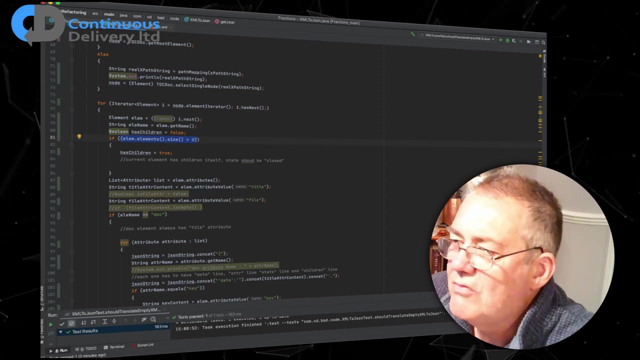 This iterator is listed over a list of elements. Well, the code tells us that, so that can go. Current element has children itself states should be closed. So has children equals, true. So we could say that if we changed that, if we named that evaluation, so if we created a method called 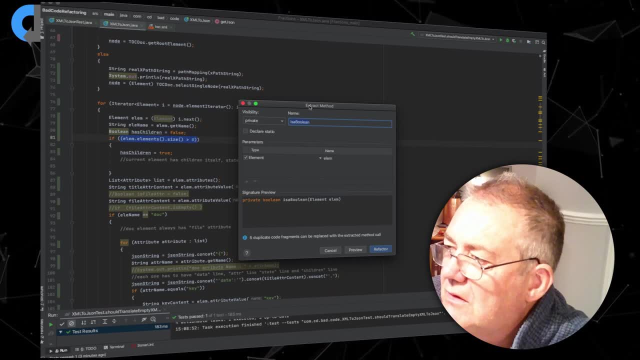 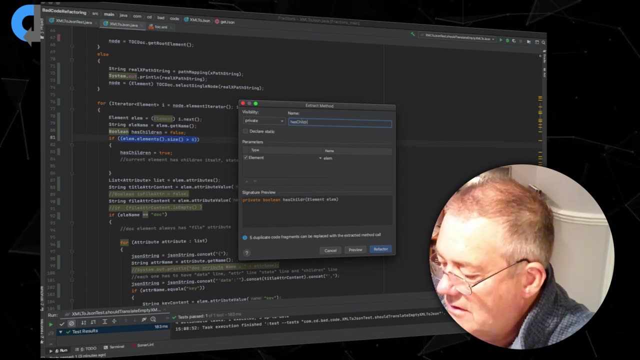 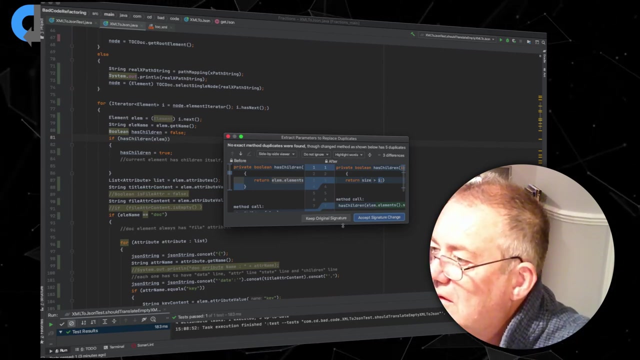 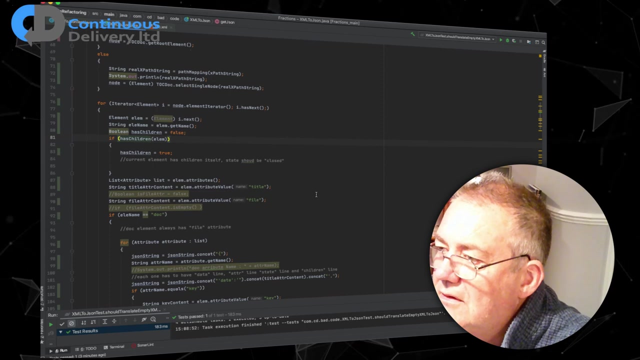 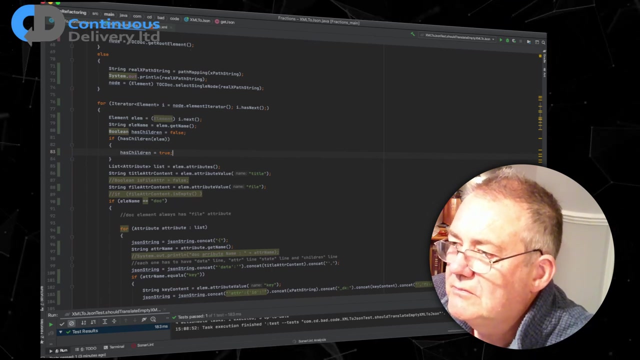 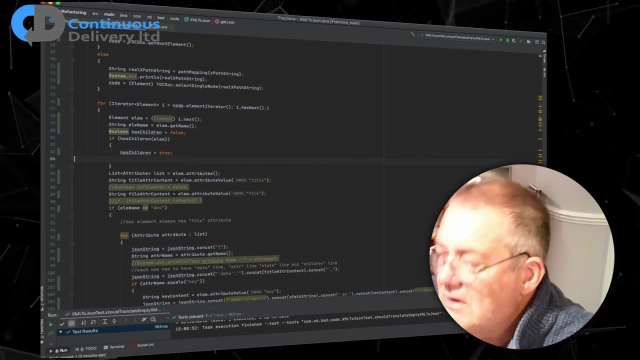 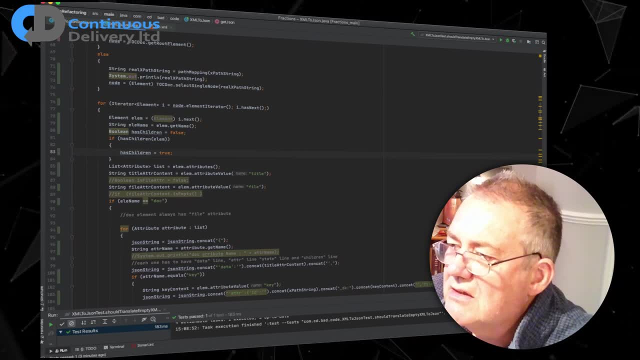 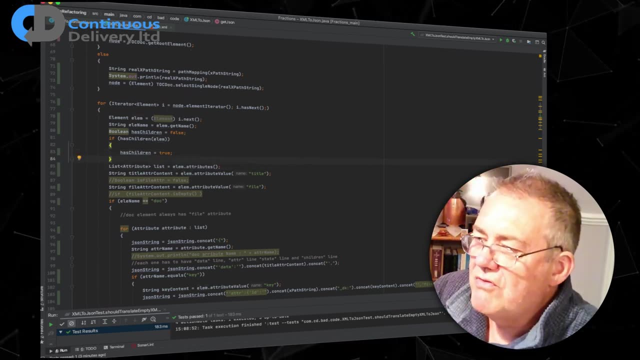 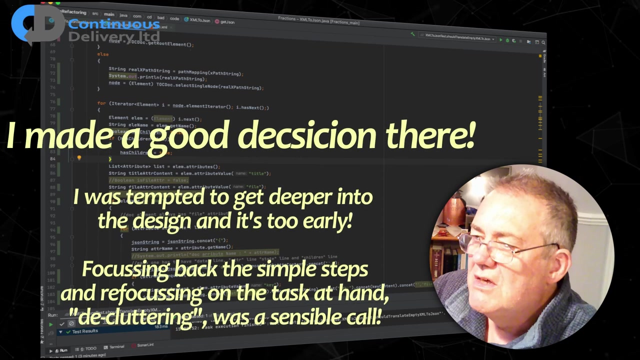 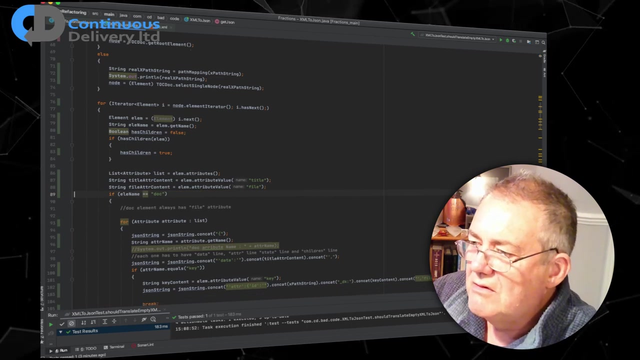 be closed. So what we're really interested in is: is the state closed? Let's come back to that for now. but because we're just removing clutter at the moment, So has children removes the need for that documentation, Well, that's just dead code. That's just dead code. Document element always has a file attribute. 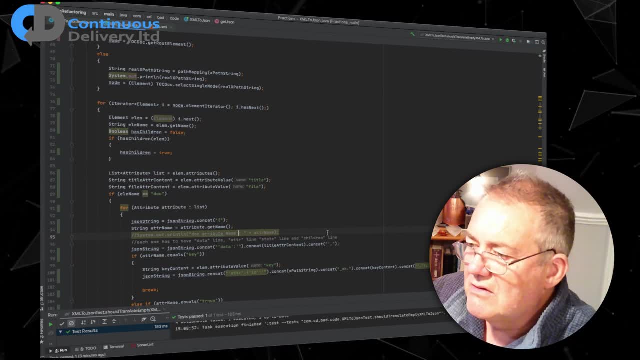 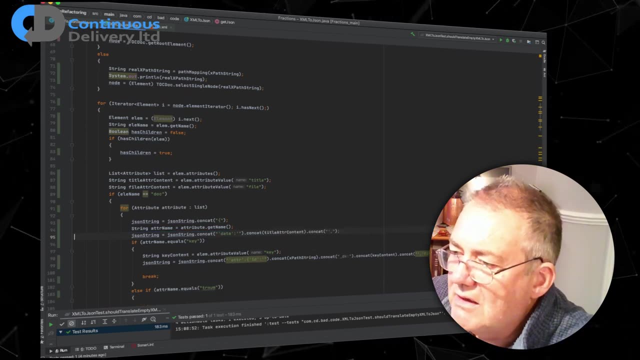 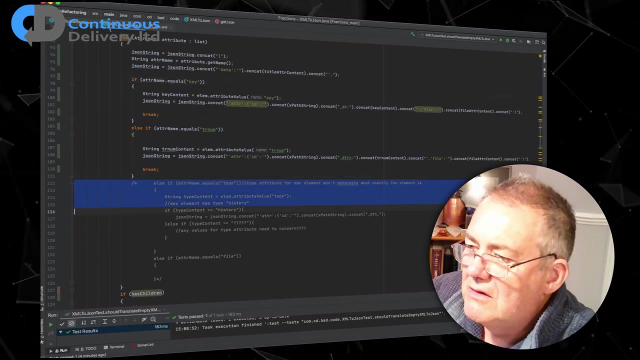 Um, that's just telling stuff. That's not very interesting. That's: each one has total data. Yeah, Um, it's not really helping, So let's get rid of it. Uh, more dead code In the real world. if I was doing this kind of thing, I would be certain that I would have uh. 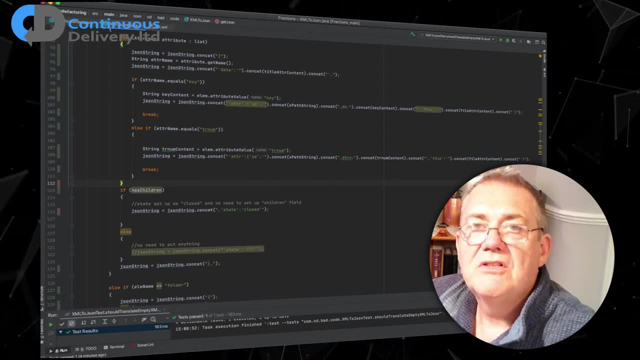 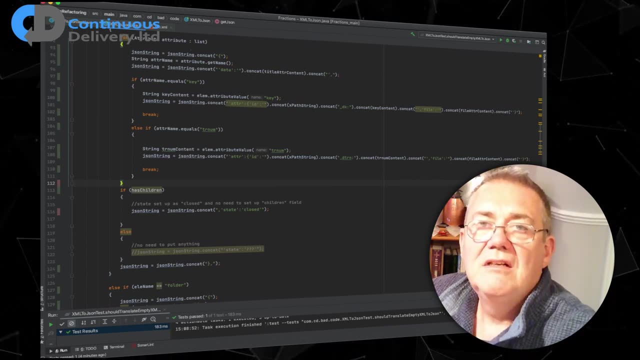 the original version in version control, the original version of the code, and I would be periodically- uh, pretty much every time I run a test, I would commit the result so that I'm at a stable point for efficiency of data. I would be able to do that. 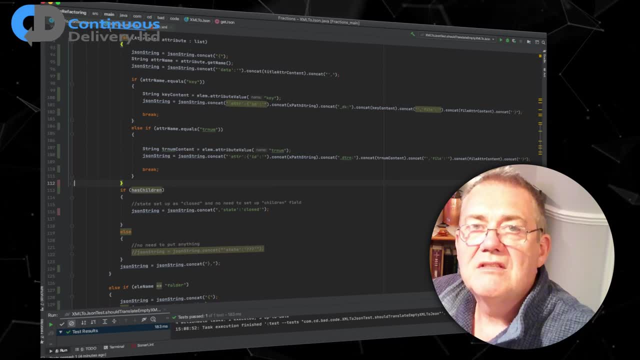 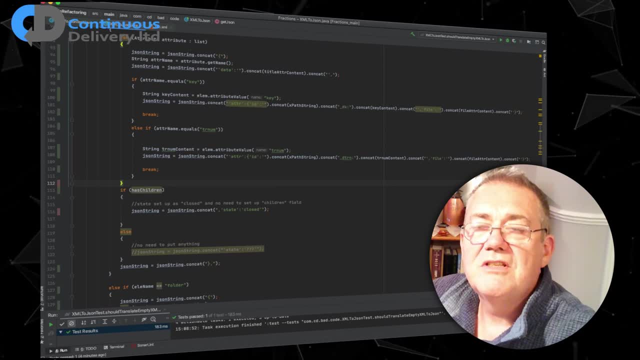 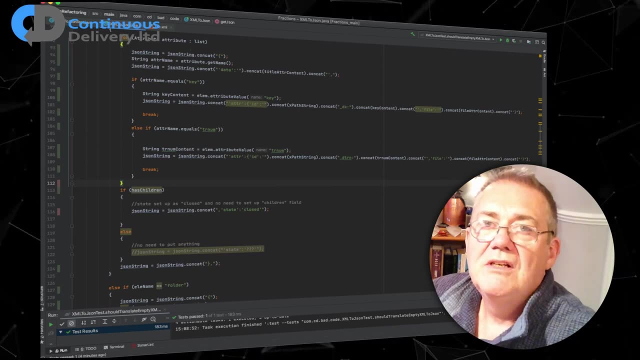 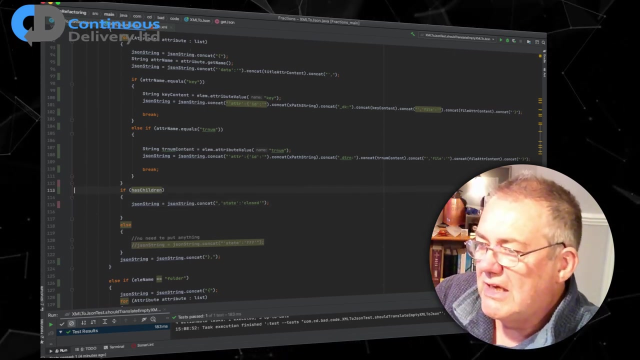 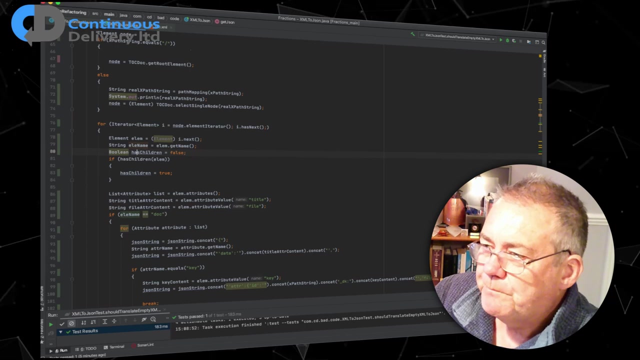 but in the real world I would be using my version control system to give me the ability and confidence to make changes and always to be able to step back to a stable position as I make progress. so here's. this has children thing again. so we've collected up here. 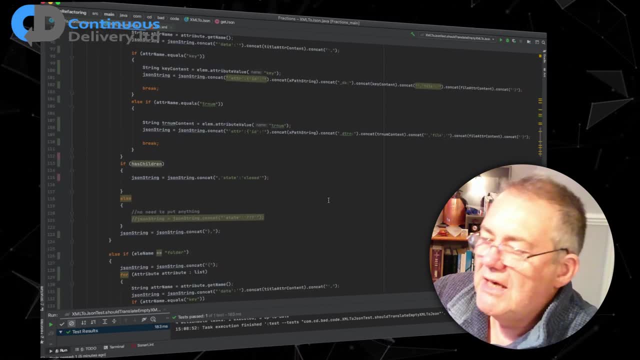 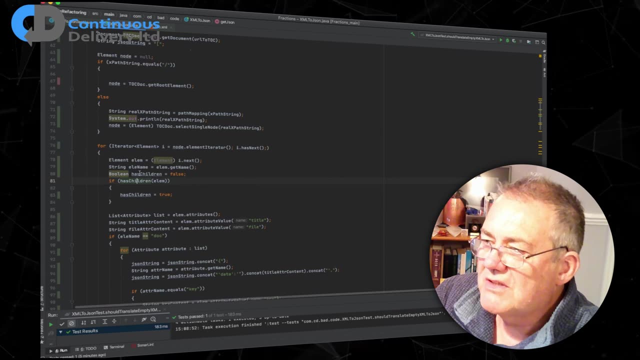 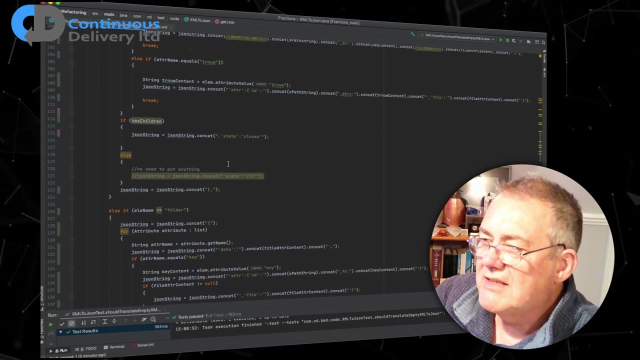 if has children. I'm going to leave that for later, but I'm spotting something here in that I I think there's no reason for us to do separate these two things out. we might as well move this evaluation down to here and just carry it out in line, and then all of this code would be a lot simpler. 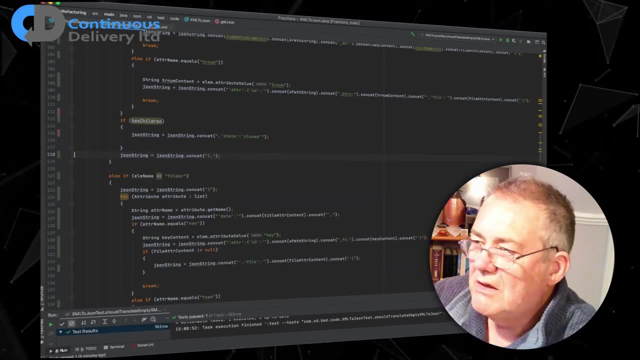 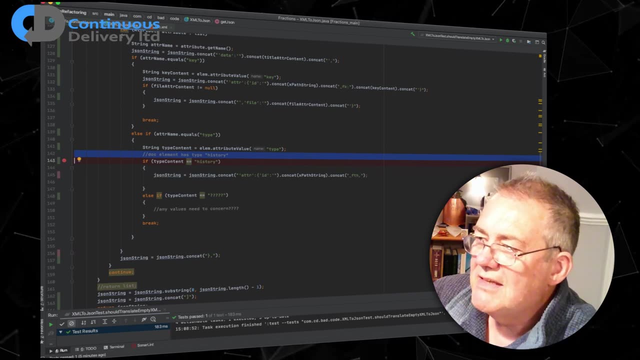 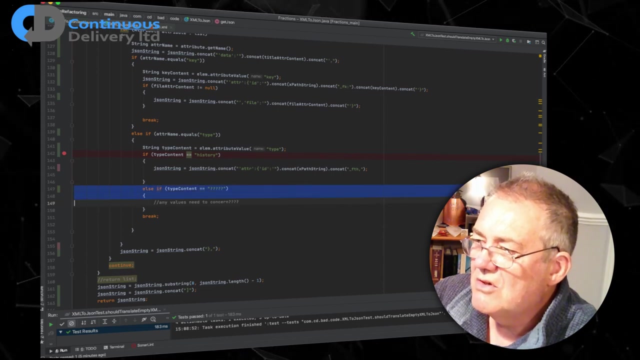 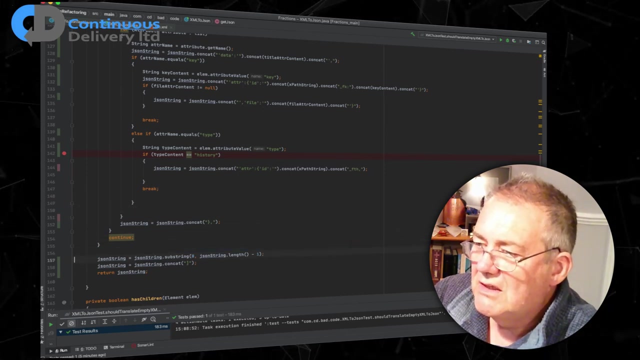 so this, all of this, is dead code. it's doing nothing, let's carry on. or if document elements, it has history and it says there it has history. else, if type content is question mark, don't do anything at all. so that's dead code. return a list. yeah, that's dead code. that's a redundant comment. read X pass. 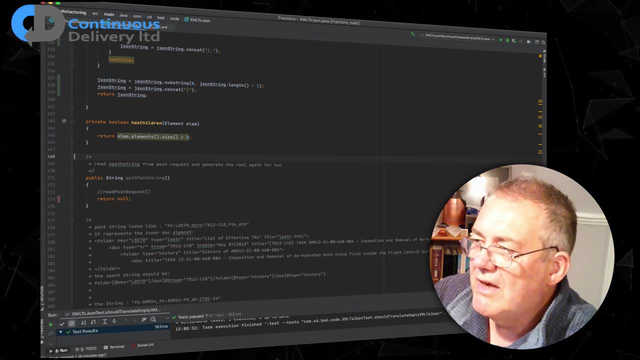 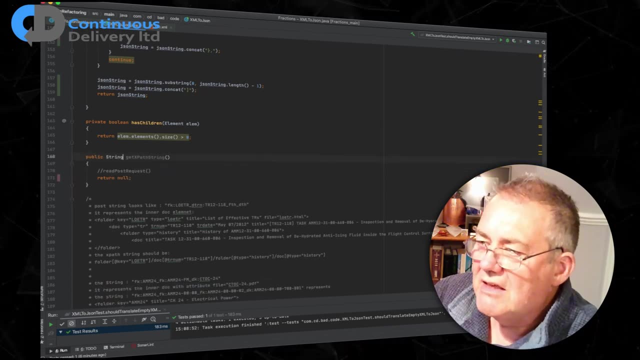 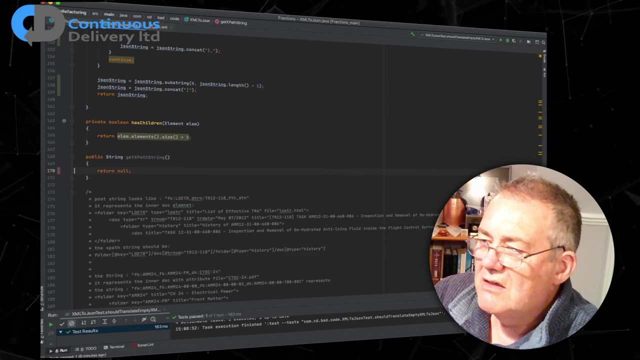 string from post request and generate the real X path for TOC. so that's actually doing nothing at all. I can't delete this because it is a public method and I don't know what's calling it, but according to this, nothing in the code that I have is calling it. I can certainly delete that because that's. 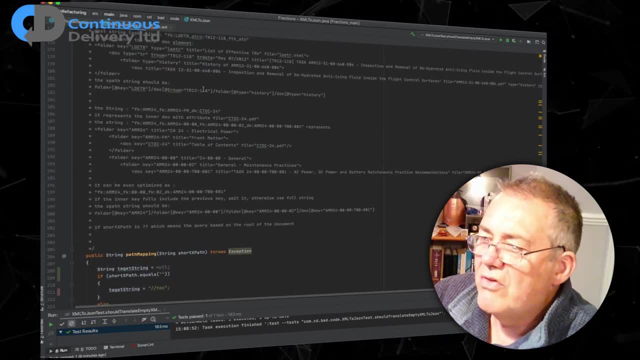 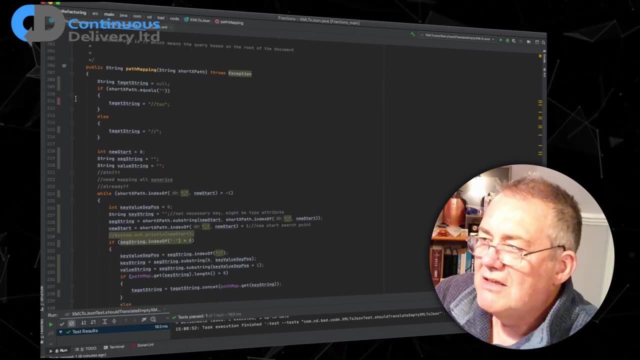 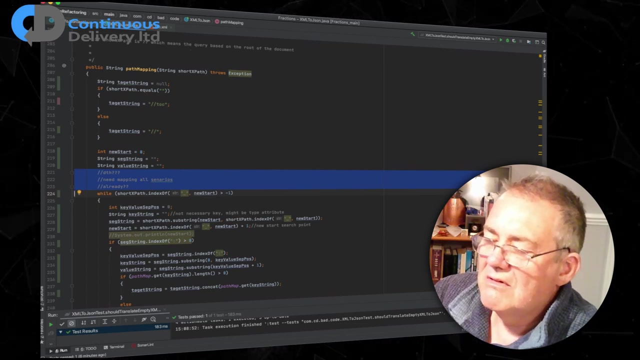 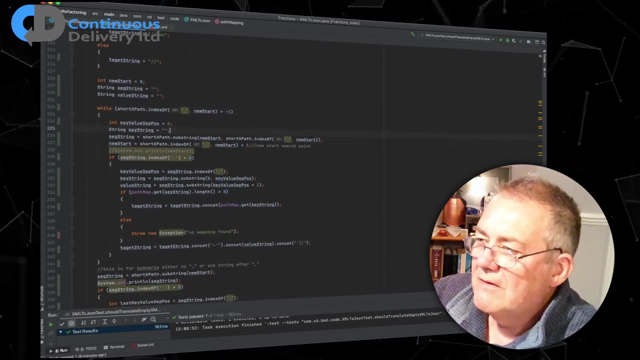 doing nothing, so this is waste as well. this is another one of those things that's. this is actually where I got the information in order to build my test input data. I'm not going to delete that right now. yeah, this is just looks like a program and just using to themselves. let's get. 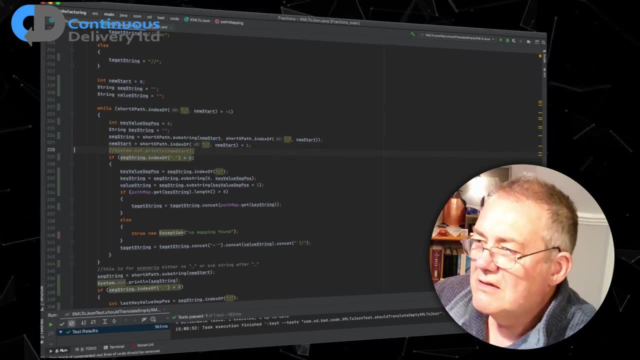 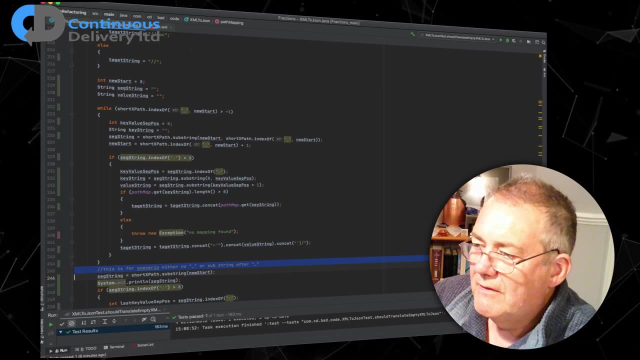 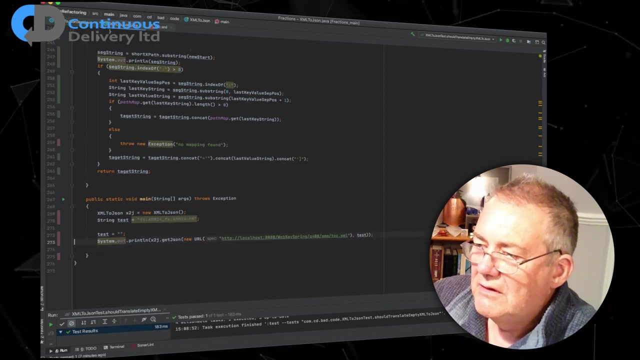 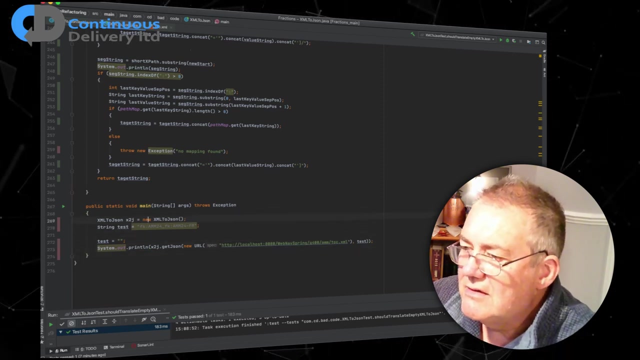 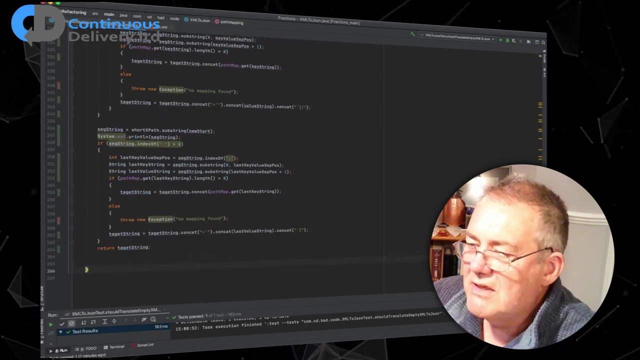 rid of that. that that, yeah, Forgive me, Thanks for watching, right? so here's, here's the main method, and actually this main method is only a test and we have a test. that's a test, so we can get will delete that main method. that's, we've replaced that with a test. so let's run our test again and make. 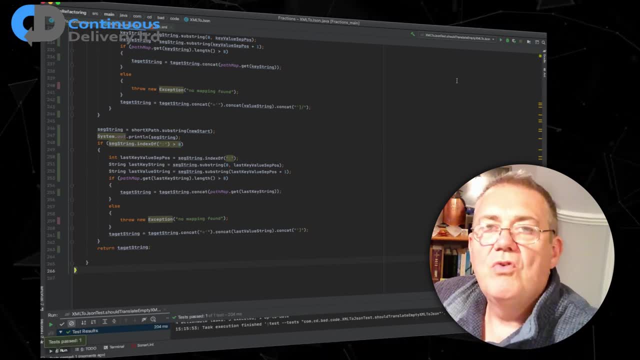 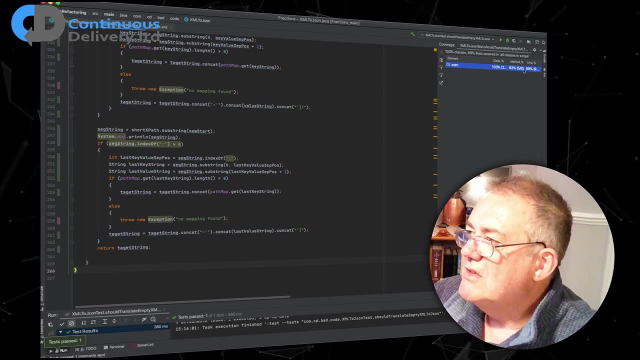 sure that we haven't broken anything. everything's good. as I said before, at this point I would commit. let me just run the coverage again, because we just made some changes and the line coverage has gone up. so now we've gone up from about 86 percent. 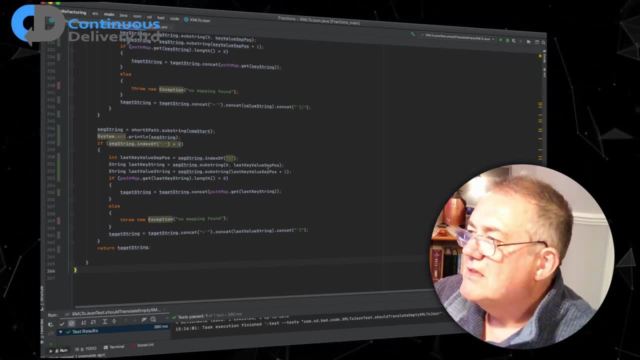 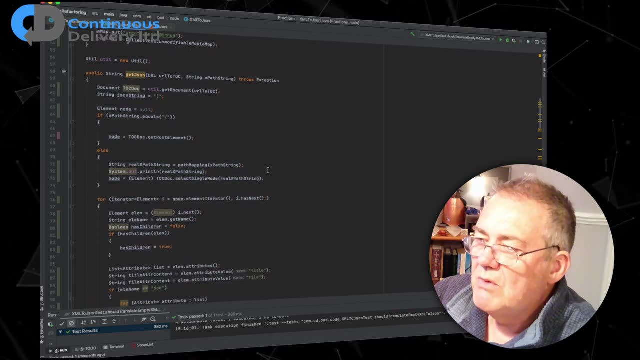 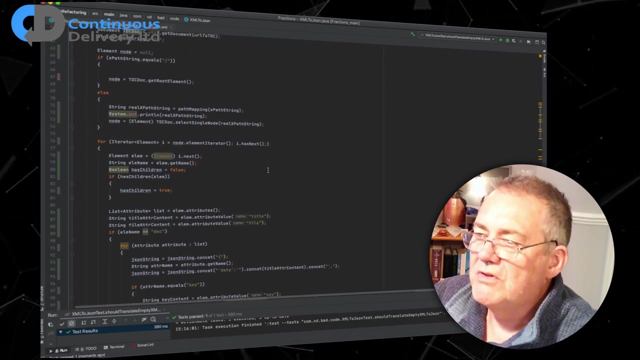 to, or 85 percent to 89 percent. so that's that's. that's a step in the right direction, right? so let's go back to our code. we're in a stable position. we, we know what's, we know that we're our code is doing exactly what it was doing before, because we've just run the approval test. 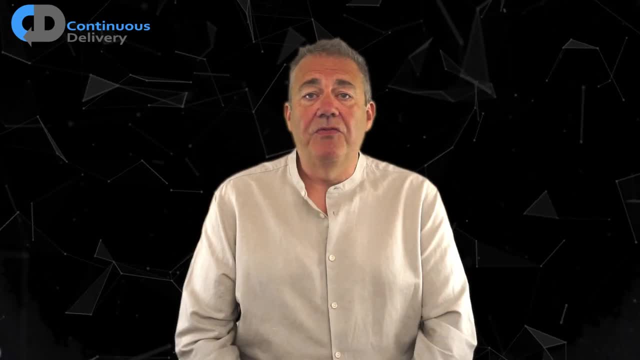 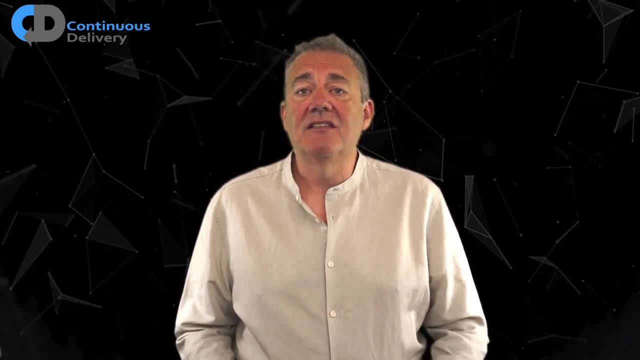 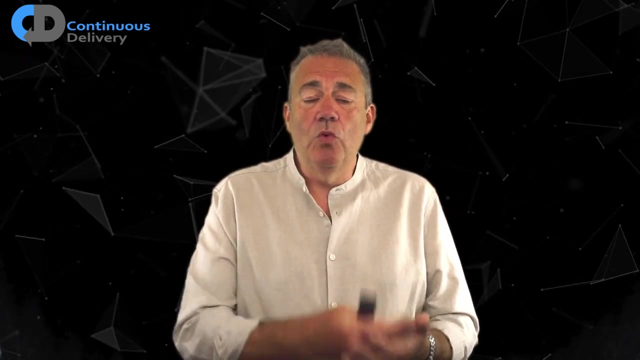 remember, the approval testing is powerful. it gives us it's simple to add to almost any code base. it gives us a strong defense against inadvertent changes to that code base and so is the perfect backboard against which we can work to to carry out with the refactoring steps that we need to. 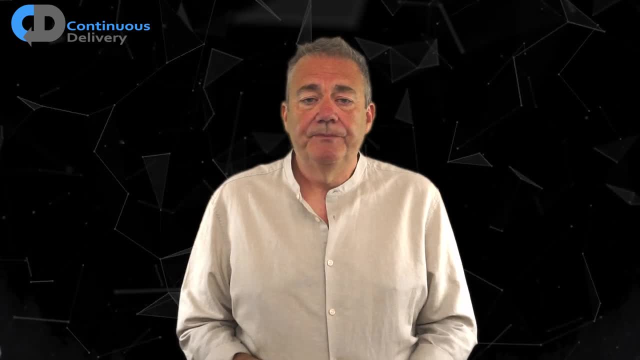 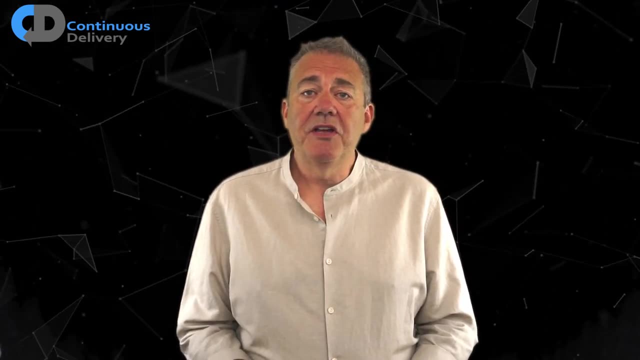 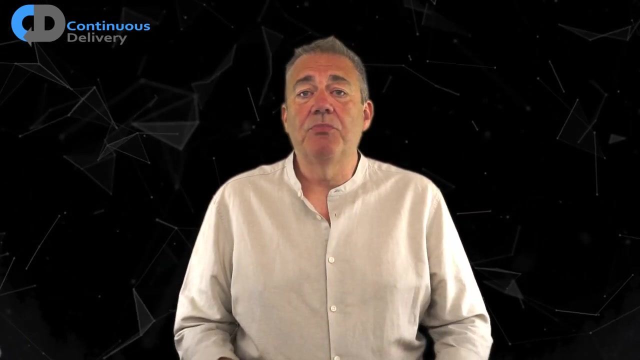 to get the ship, the code into a more workable shape. removing clutter is also important. it makes the structure of the code that we're working in much more obvious and therefore it makes it easier for us to spot those changes that we can make to improve the improve the code. 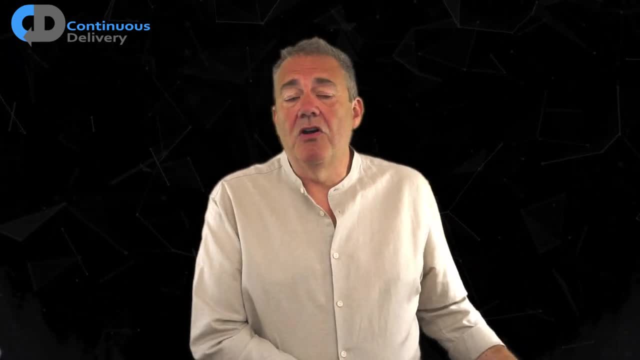 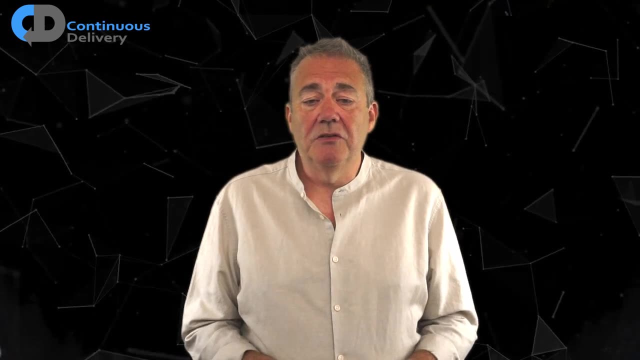 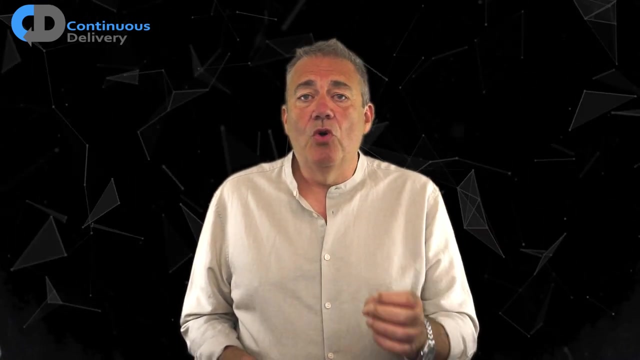 remove the dead code. keep, have a version control as a backup, but remove the dead code and then you will get much better visibility into the structure of the code. and the last and most important of these are pieces of advice, for refactoring is working: small, tiny steps into the code.